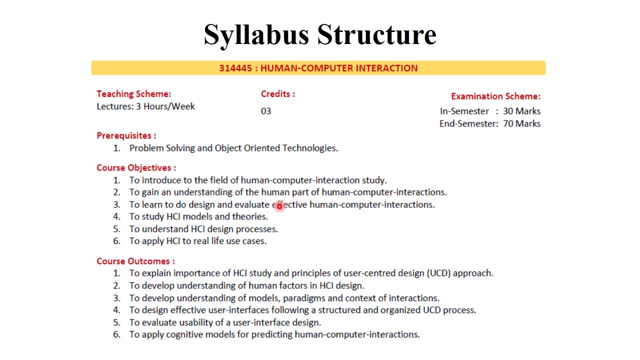 part of human-computer interaction. We will also learn about design, evaluate effective human-computer interaction and also study of different SCI models and their theory and to understand the SCI design process. and we also learn about SCI in real-life use cases- Okay, because each and every field nowadays computers are used, So there are more real-life. 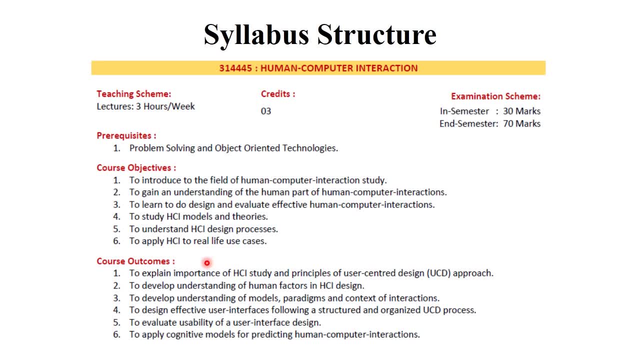 examples are appeared in that subject. The course outcome is to explain importance of SCI study and principles of user-centered design approach, to develop understanding of human factors of SCI design and also to develop understanding of models, paradigms and context of interaction, and also to design. 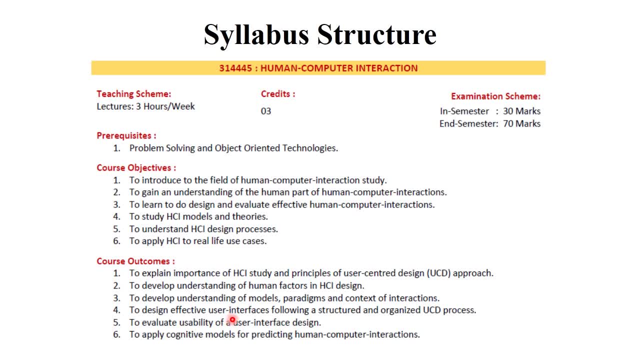 effective user interface following a structured and organized UCD process. From this subject to evaluate usability of user interface design. User interface design generally use each and every IT department or each and every software company, So we will learn about this user interface design process. and also to apply cognitive models for predicting human computer. 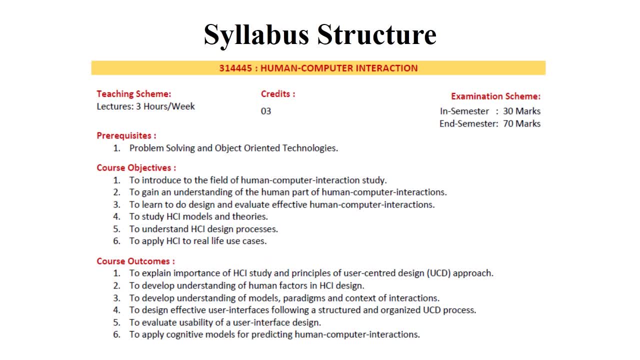 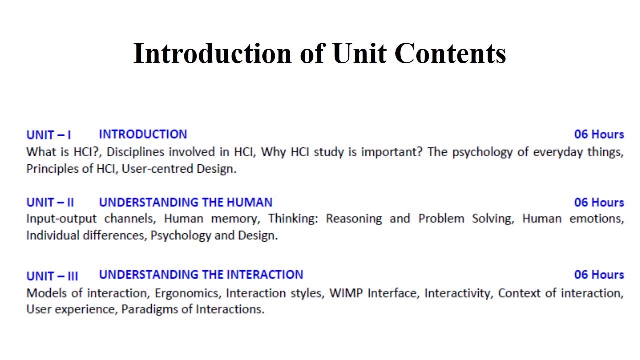 interaction. Okay, so this is the course objective and course outcome. That is why this subject involves in your syllabus. Okay, Introduction of unit contents. The first unit is introduction. In this unit we will learn about what is human-computer interaction. So first of all we will learn about what. 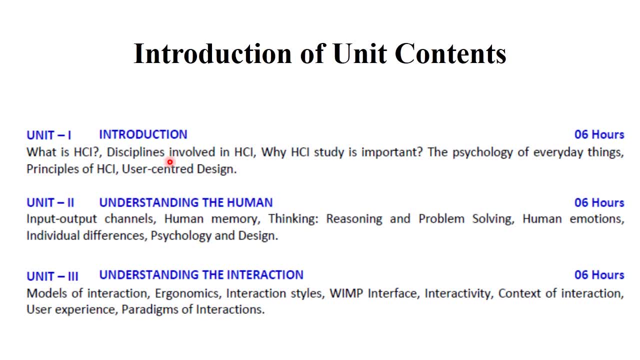 is human-computer interaction. In this unit we will learn about what is human-computer interaction, the goals, benefits of human-computer interaction- okay, and also there are various disciplines or fields which involves HCI. that is, human computer interaction. okay. we will also learn about user-centered design process. 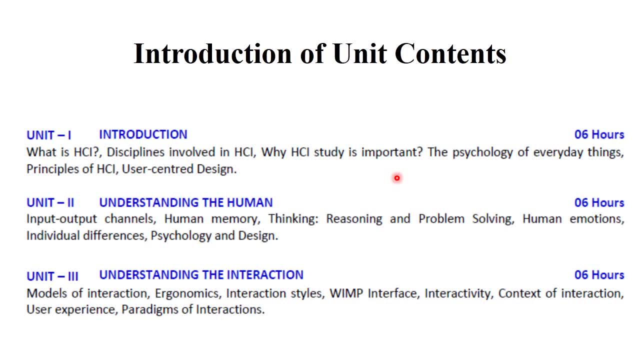 principles of HCI and the psychology of everyday things. this is your first unit. in first unit we will learn about each and every introduction of HCI. okay, the next second unit, the human-computer interaction, means there are total three words: human, computer and interaction. and these are again and next three units. 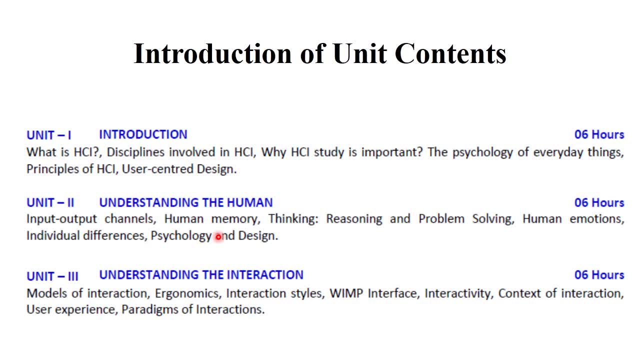 that is human. next unit is computer and next unit is interaction. okay, we will learn in deeply how exactly human is interacted with computers and computers is interacted with the human. clear now. the second unit is understanding the humans. in this unit, we will learn about input output channels. 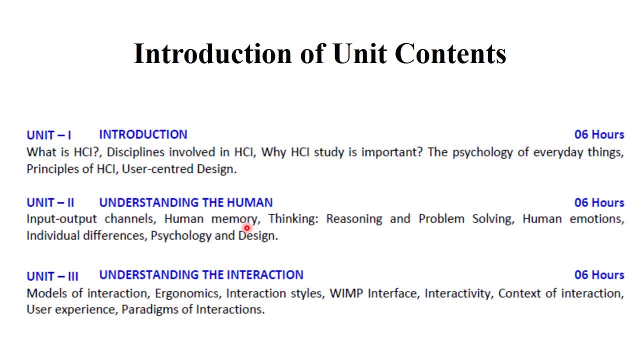 the human memory. there are various types of human memories where informations are stored, then thinking and reasoning and problem-solving. the human emotions- there are various emotions- are includes in human, then individual difference, psychology and design. this all points are involved in understanding the human. so we understand the human by using these points or by 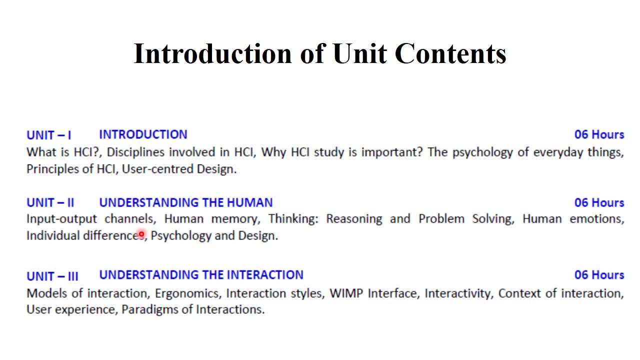 using computer interactions. clear, okay. the next third unit is to understanding the interaction. in this unit we will learn about models of interaction. there are different models of interaction: ergonomics, interaction style. we all are familiar with this interaction style, but we will learn in deep way how exactly. 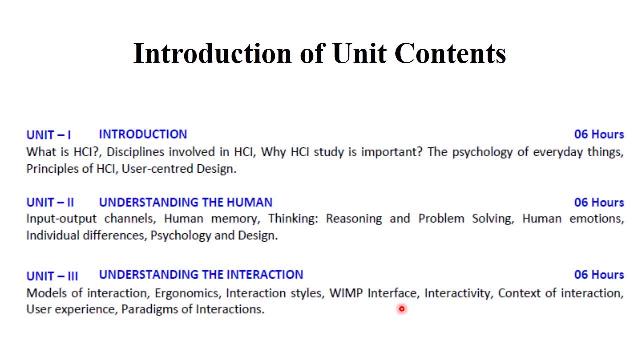 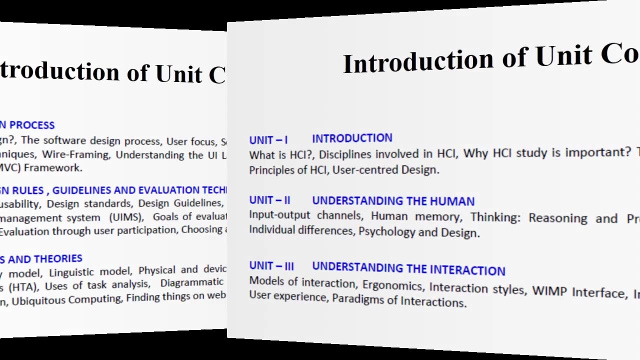 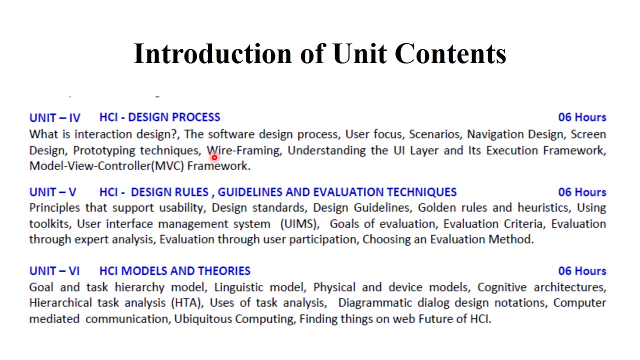 interaction styles are work, then WMP interface, then interactivity, context of interaction, user experience and paradigm of interaction. okay, so this. all points are involved in understanding the interaction here. okay, next fourth unit is HCI design process. in this unit we will learn about what is interaction design, the complete software design process, mostly the some. 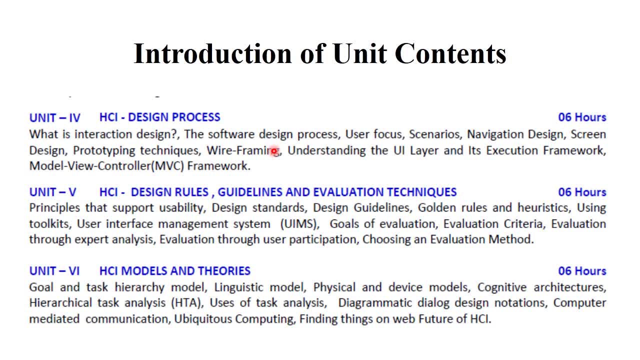 students are familiar with software development life cycle, right, so this is software design process. we will learn deeply in the form of computer interaction. then user focus scenarios, navigation design, screen design, prototyping technique, then wire framing and understanding, user interface layers, execution- same work and model view Commentary. okay, in real. 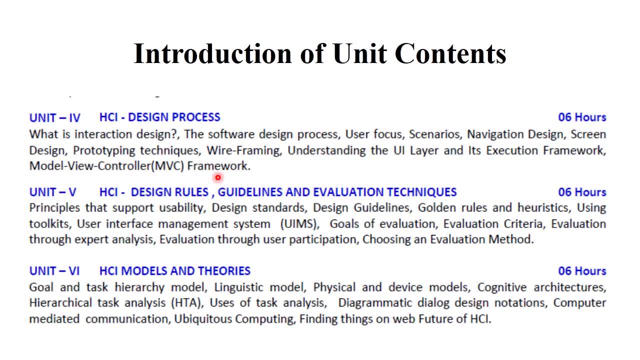 life we use all these things, but it doesn't know the what exactly mean that okay, so in this video we learn these all things in the anyway. the next unit is HCI: design rules, guidelines and evaluation techniques. this unit contains principles that support usability, design standards, design guidelines. there are some also golden rules and heroes tricks using. tools- nothing free destination standards, design guidelines in the process. there are some also golden rules and heroes, tricks to build and answer the market, and other things. there are plenty more things available in this signature. this unit best Mitarbeiter has in termsω available as well as tools to use when you want to perform any work. 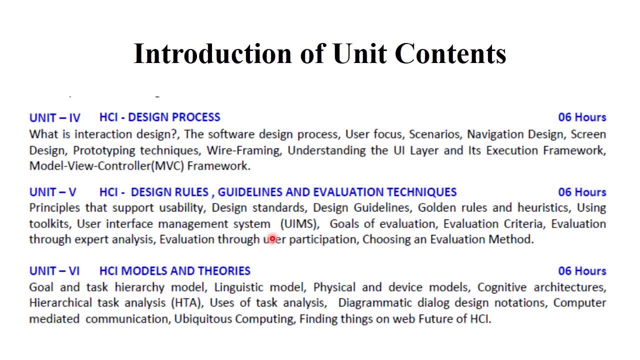 metrics using toolkits, user interface management systems. then goals of evaluation, evaluation criteria, evaluation through expert analysis and evaluation through user participation and choosing an evaluation methods. okay, So these all points are used in industries: how to develop the product, how to develop? 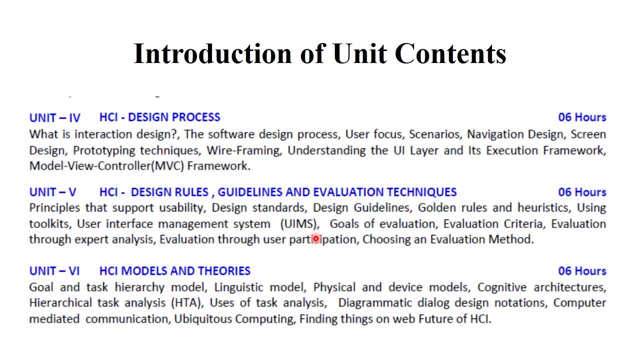 interactive design, okay, and how to involve the users in that particular project. So these all things we learn in that particular content or of unit, okay. And the last unit is HCI model and training. There is a goals and task hierarchy model: linguistic model, physical and device model. 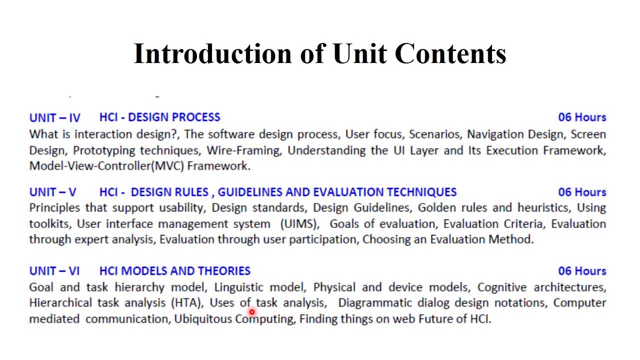 cognitive architectures, then hierarchical task analysis, uses of task analysis, diagrammatic dialogue, design, notation, computer mediated communication, ubiquitous computing and finding things on the web, future of HCI- okay, So these all things are involved in HCI models and training. okay. 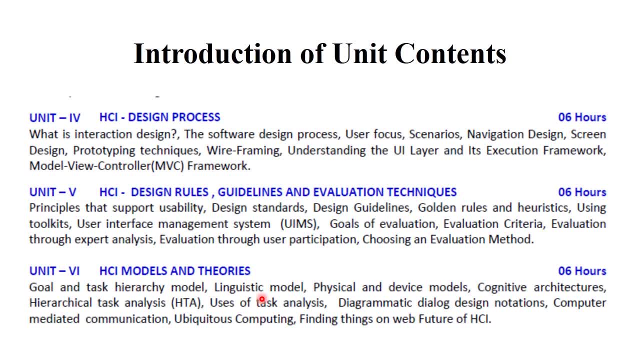 So HCI, that is, human computers interactivity. This term use each and every field, whether it is technical field and non-technical field. okay, So this subject is more interactive subject. okay, So this all points. we will learn step by step. 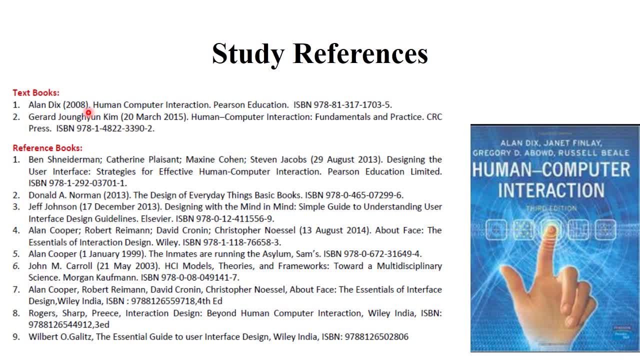 There are some references. okay, So there are some text book references and references book. So I will suggest you. you used Alan Diggs. that is author Alan Diggs. the book name is human computer interaction and peer learning And peer self education. this book 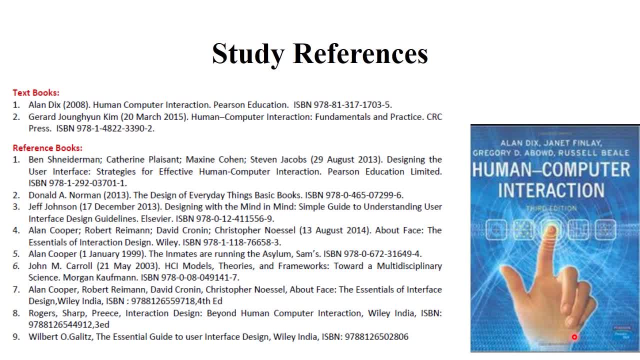 This is the front structure of that particular Alan Diggs book. This book involves each and every points in more deep way. Some students or some of the peoples have more interest in human computer interaction for further study and for research purpose. then you need to use this book. 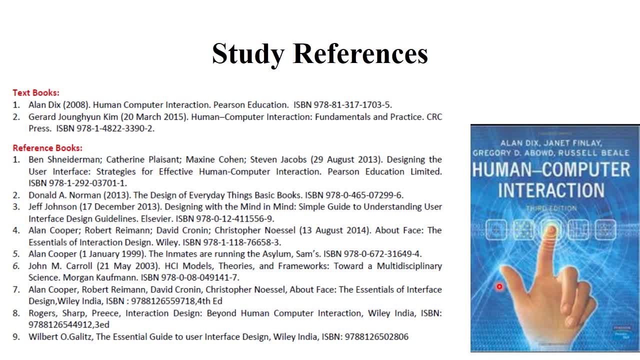 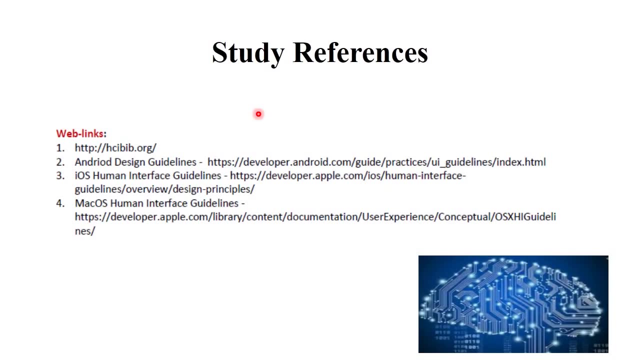 It is a very good book for reference purpose, okay, And also I will explain through my videos each and every points in more detail. Okay, So you can use this example way or more in detail way, okay. Now these are the some study references by using web links, okay.